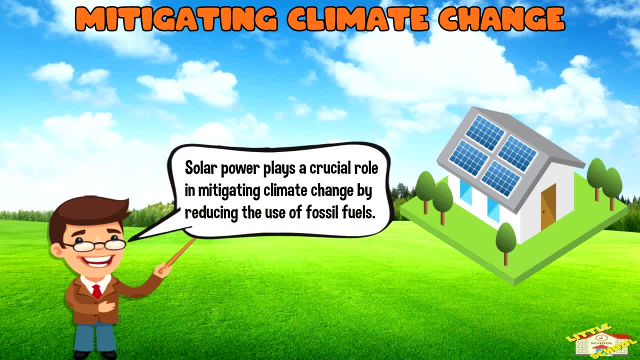 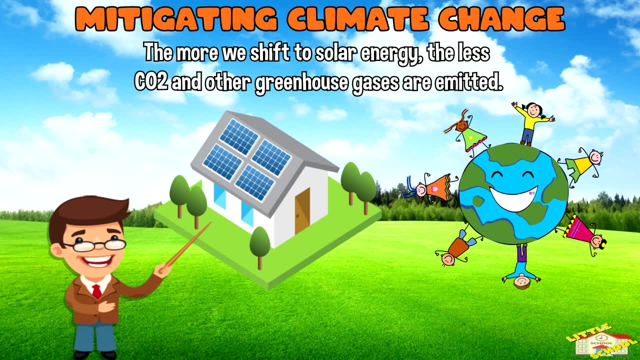 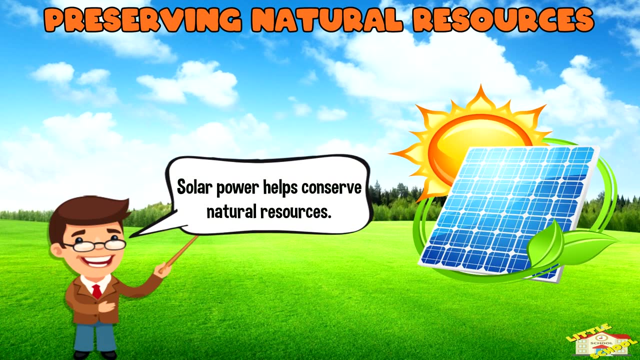 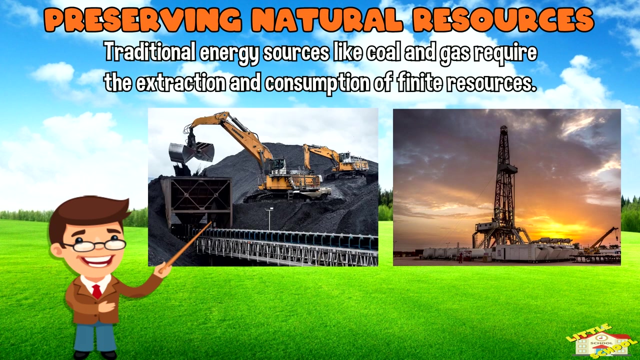 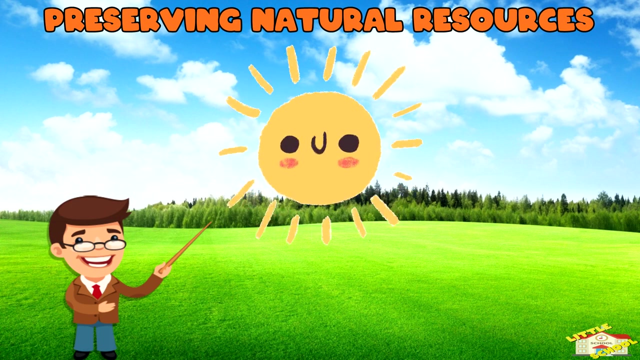 The more we shift to solar energy, the less carbon dioxide and other greenhouse gases are emitted. Preserving natural resources: Solar power helps conserve natural resources. Traditional energy resources like coal and gas require the extraction and consumption of finite resources. Solar energy, on the other hand, utilizes unabundant resources. 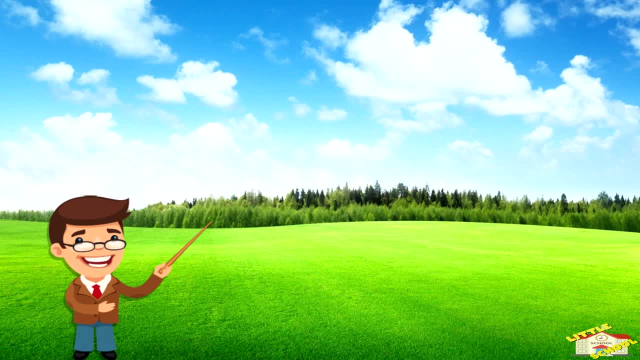 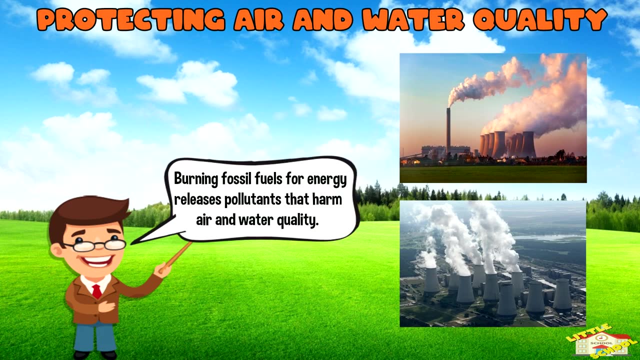 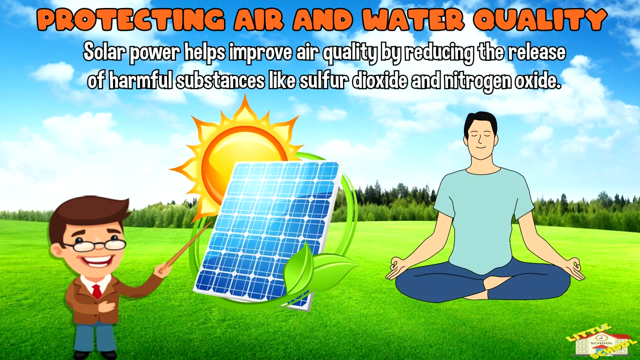 The sun, Protecting air and water quality. Burning fossil fuels for energy releases pollutants that harm air and water quality. Solar power being clean and emission-free, helps improve air quality by reducing the release of harmful substances like sulfur dioxide and nitrogen oxide. 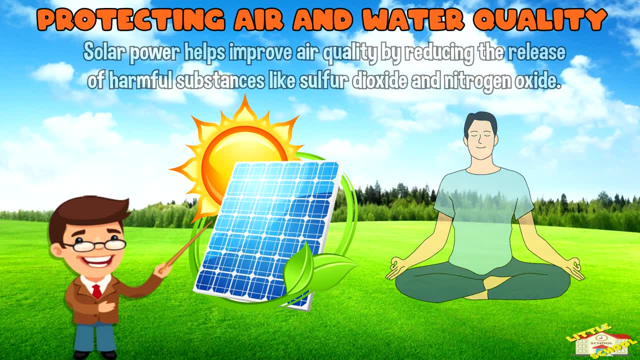 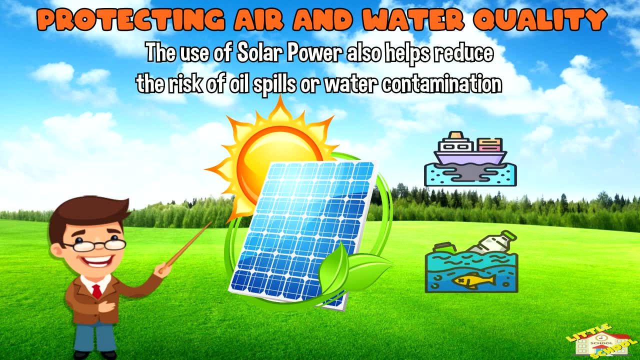 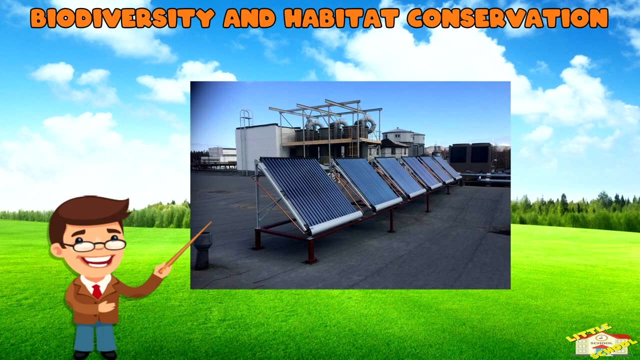 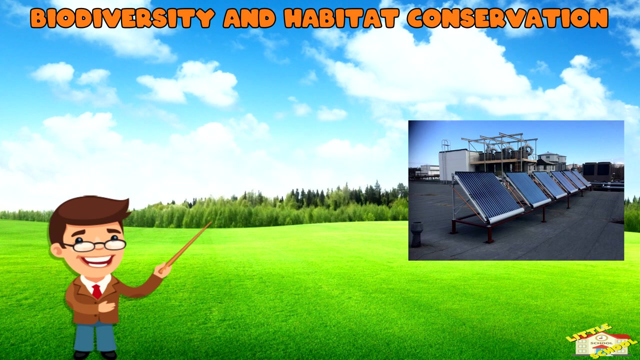 Solar power helps reduce the release of harmful substances like sulfur dioxide and nitrogen oxide. The use of solar power also helps reduce the risk of oil spills or water contamination associated with fossil fuel extraction, Biodiversity and habitat conservation. Solar power installations take up relatively small amounts of land. 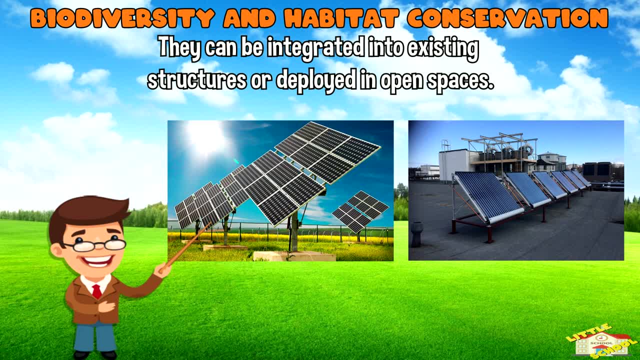 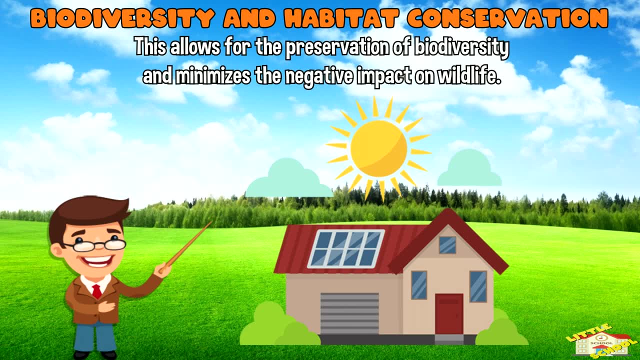 They can be integrated into existing structures or deployed in open spaces without causing significant disruptions to natural habitat. The use of solar power helps reduce the risk of oil spills or water contamination associated with fossil fuels. This allows for the preservation of biodiversity and minimizes the negative impact on wildlife. 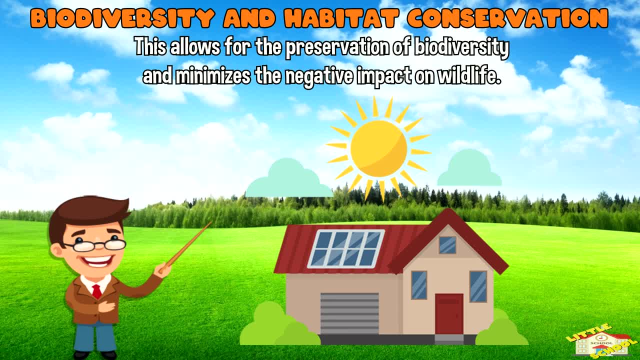 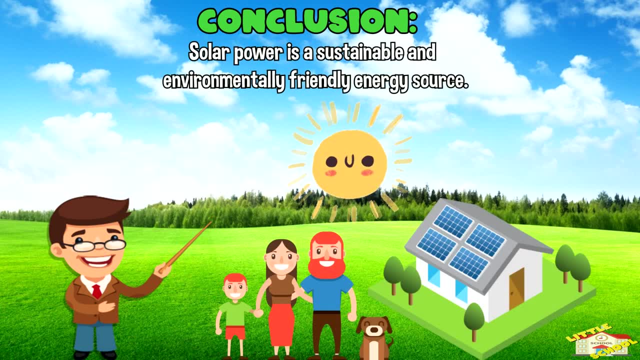 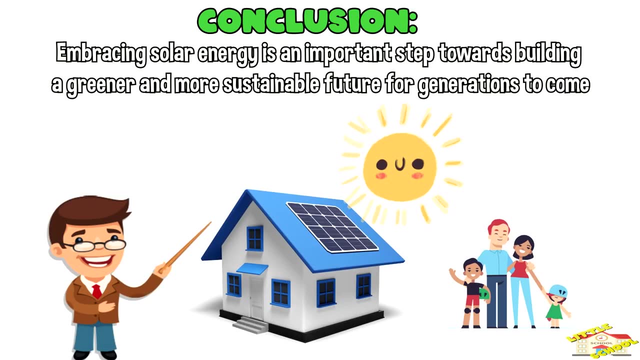 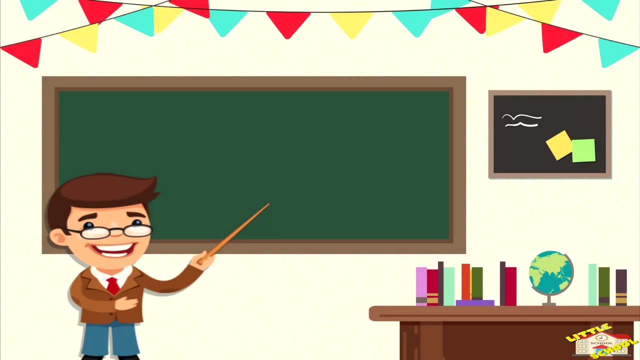 compared to other forms of energy generation. In Conclusion, Solar power is a suitable and environmentally friendly energy source. Embracing solar energy is an important step towards building a greener and more suitable future for generations to come. And that is all for today's video. I hope you enjoyed learning about the impact of 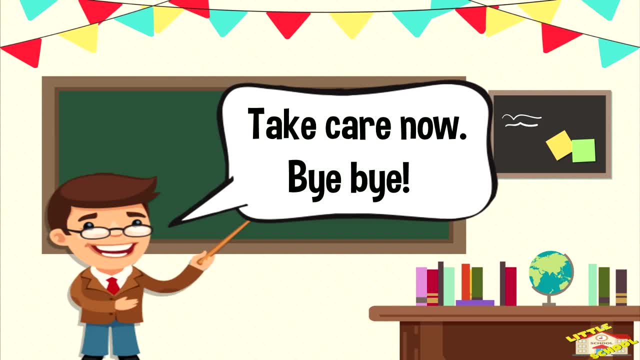 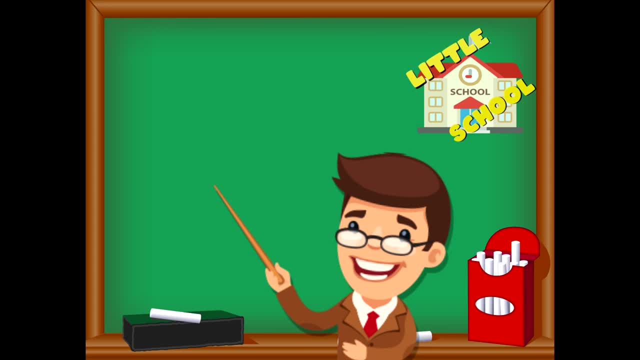 solar power on the environment today. Take care now, bye, bye. If you enjoyed the video and want to see more videos from us, please click the subscribe button. Also, give us a like. that will help us. We thank you so much and we do hope that you enjoy our videos. See you soon.